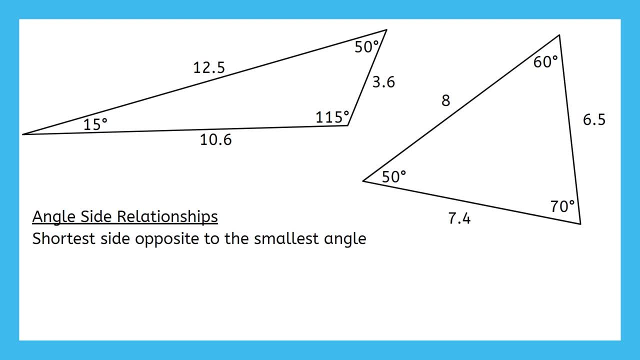 smallest angle in each of these triangles and place it on the correct side of the triangle. Here's another example of the shortest side of the triangle. Is the shortest side of the triangle directly across from them. Yes, 15 degrees is the smallest angle in the first triangle. 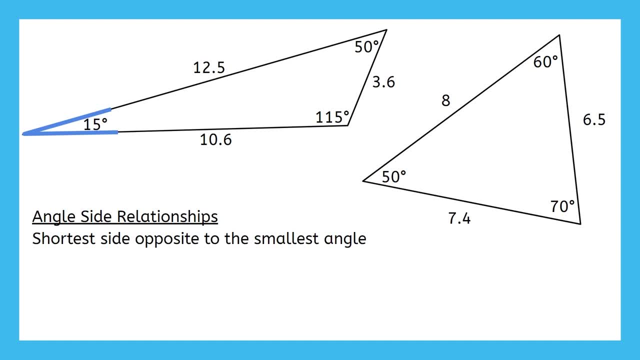 and 3.6 is the shortest side in the first triangle and they're opposite to each other. And in the second triangle, 50 degrees is the smallest angle and it's opposite to 6.5,, which is the shortest side of this triangle. Take a moment to pause the video here and convince. 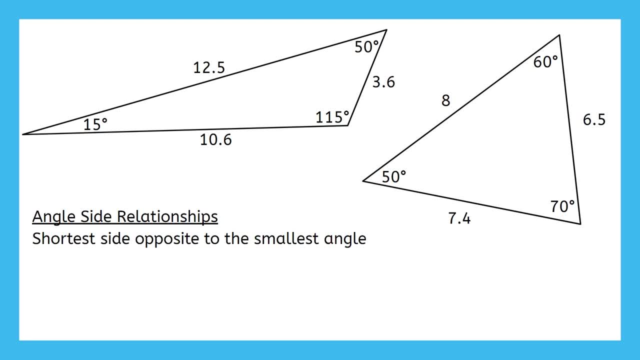 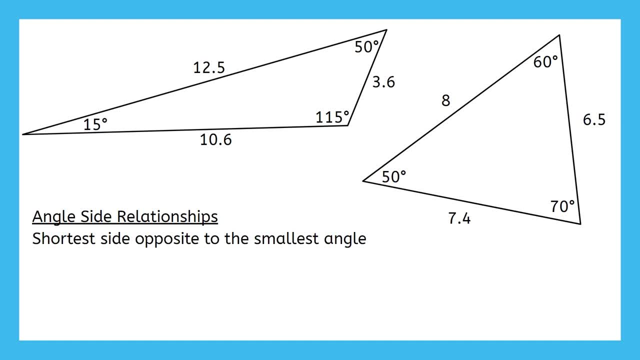 the shortest side. The same is true for the largest angle in the longest side. The largest angle in the first triangle is opposite to the longest side, And the same is true with the second triangle Also, we can go in both directions. So if I give you the longest side, you would know that it's a cross from the biggest angle. 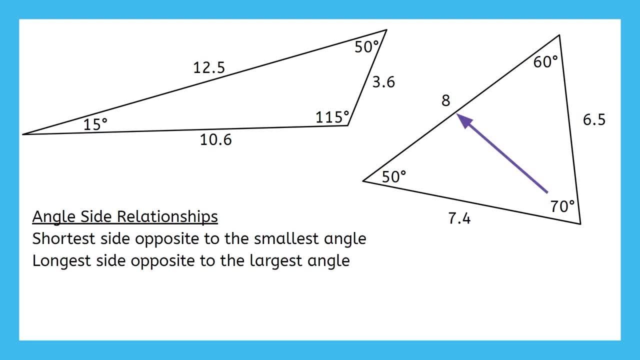 And if I give you the biggest angle, you would be able to say it is a cross from the longest side. We're going to do one example problem next, so pause the video here if you need any time to catch up in your notes template. 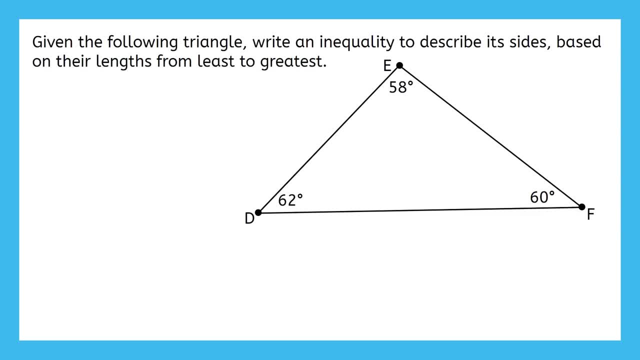 This problem says to write an inequality to describe the sides of the triangle based on their lengths, from least to greatest. Now remember that the triangles you see will not always be drawn to scale, so we need to make sure that we're applying the relationship that we just learned to solve this. 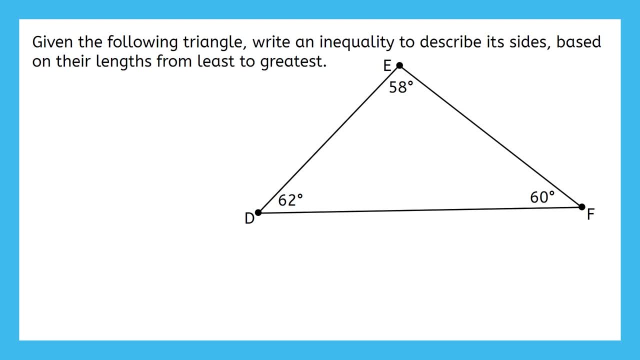 What side do you think is the shortest side? Here's the smallest angle, so the shortest side will be directly across from it. So what's the shortest side? What's the shortest angle? Well, if we're supposed to order the sides from least to greatest, let's write this side.